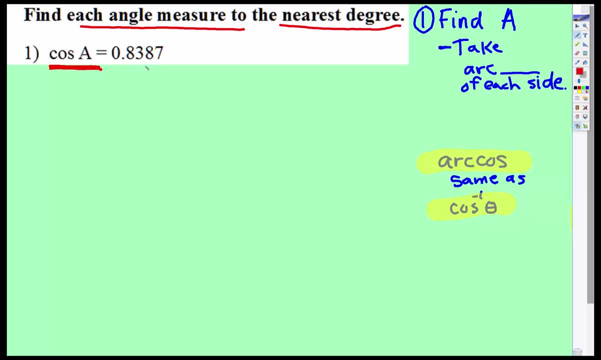 is equal and they give you this decimal answer. you need to figure out what the original theta is. So these are the steps: Find a is by taking the arc of each side, and this is what the arc sine is. Arc cosine means the same thing as the inverse of cosine, So I'll show you what that. 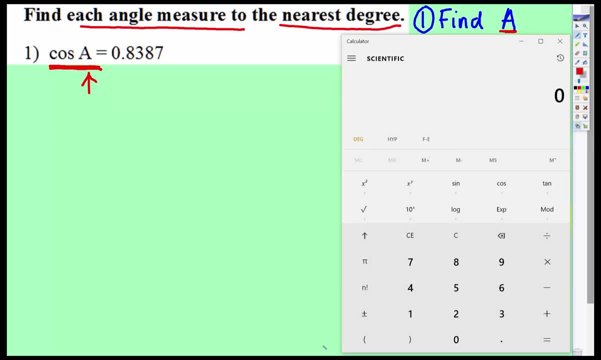 looks like on a calculator. So on a calculator, this is what you'd be doing. You'd be typing in point oops, let me clear that 0.8387, and then I'm going to hit the up arrow key. it's like the shift key on most calculators. 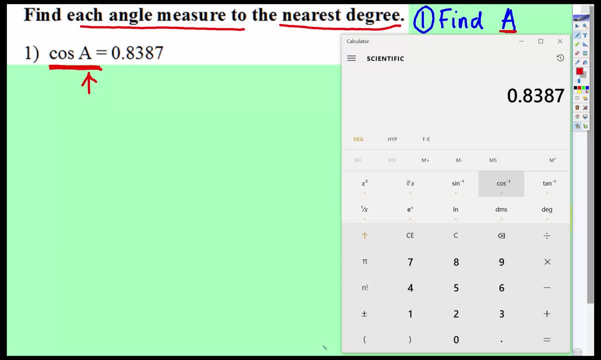 and see where it says cosine negative 1? That means the same thing as arc cosine and some professors like arc cosine, some like this. So you're going to take the decimal right here, you click that and then look at. look at what we have right there. 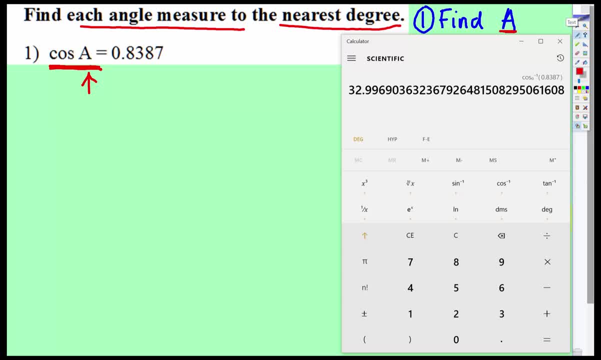 We have 32.996, but if we were to round that up, let's go ahead, and I'm going to. if you round that up, you get 33 degrees. So in this case you're going to be taking the arc cosine of each side. 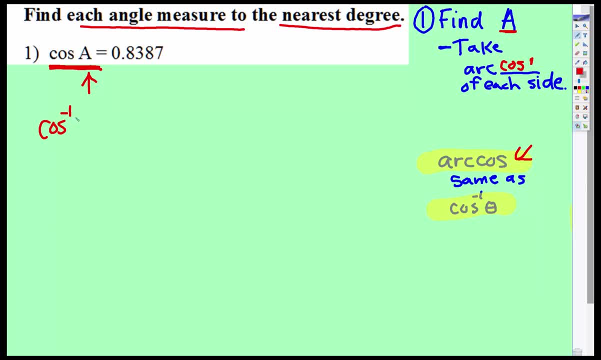 So this is what that would look like. You would say: cosine negative 1, of cosine A equals cosine negative 1, of 0.8387.. Now, if you have a Texas a T130, like we do in our classroom, 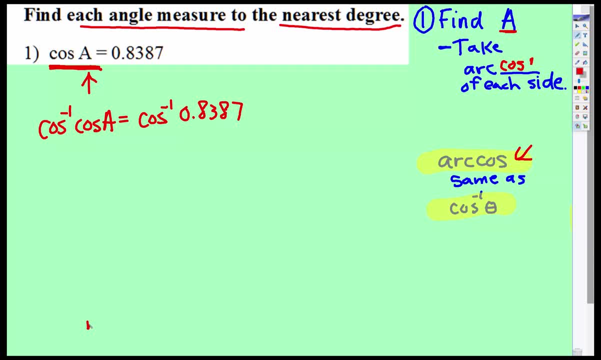 you're going to do it a little bit differently. You're going to hit the second button, then you're going to type: hit the cosine button and then you're going to type 0.. différentes 8387, and it will give you that 32.996 and a bunch of other numbers. so the